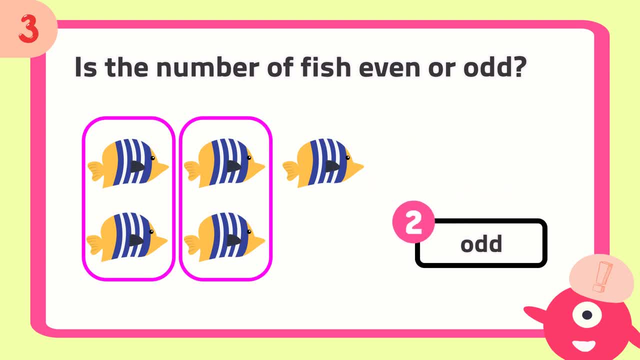 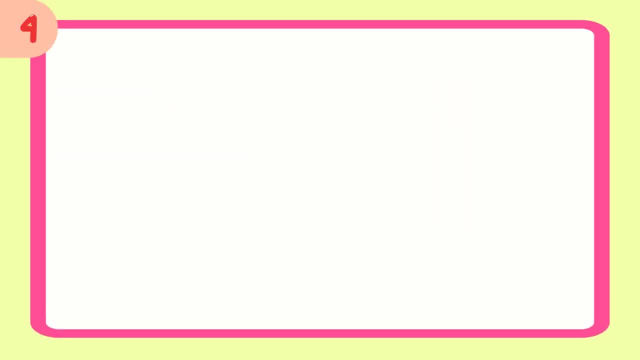 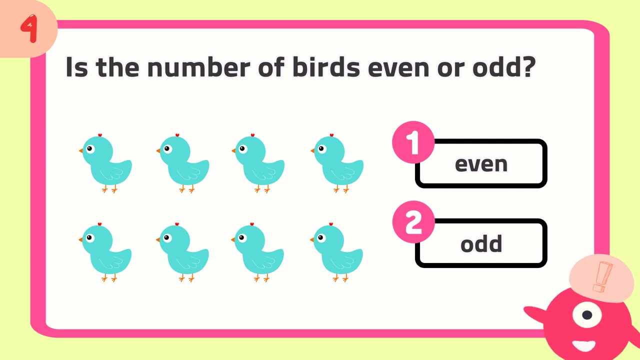 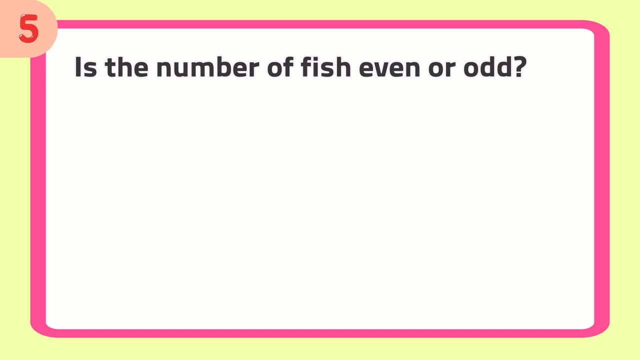 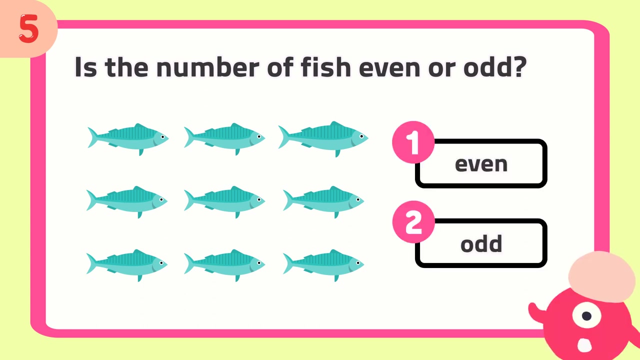 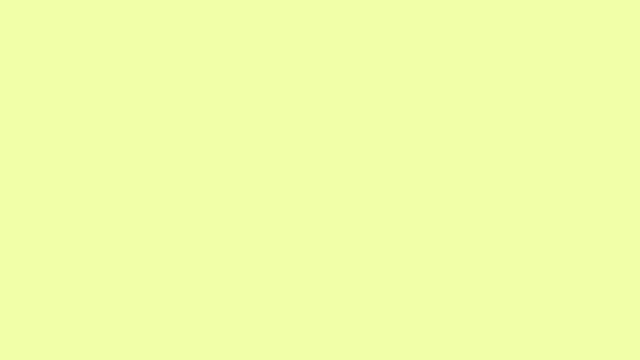 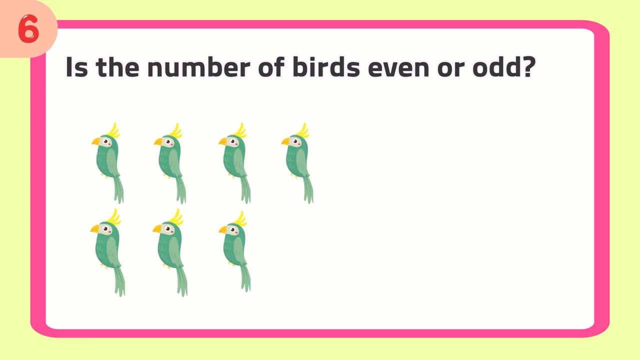 Odd Number 4: Is the number of birds even or odd? The answer is Even. Number 5: Is the number of fish even or odd? The answer is Odd. Number 6: Is the number of birds even or odd? The answer is Odd Number 6. 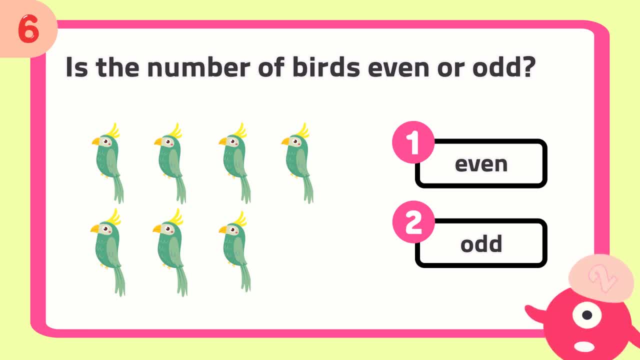 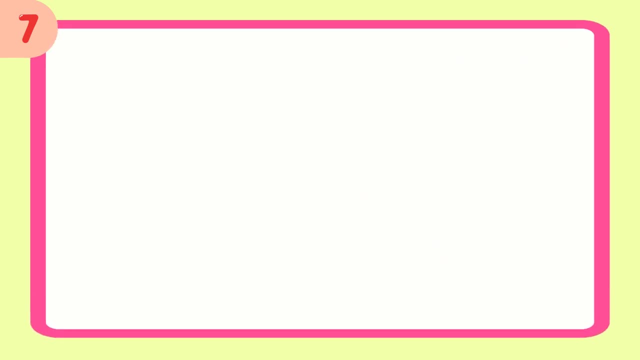 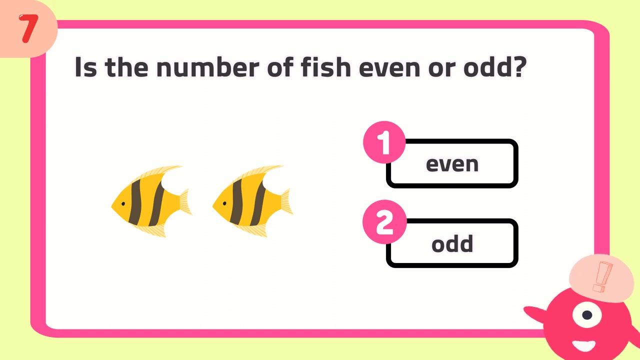 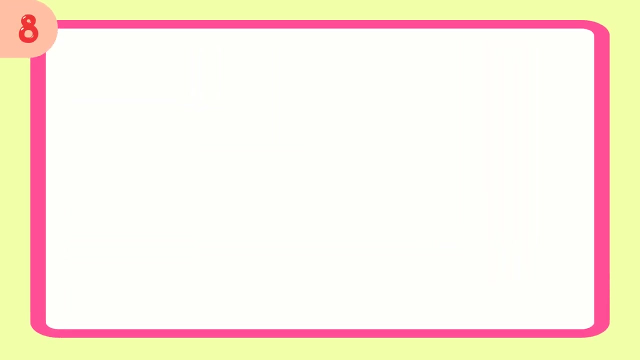 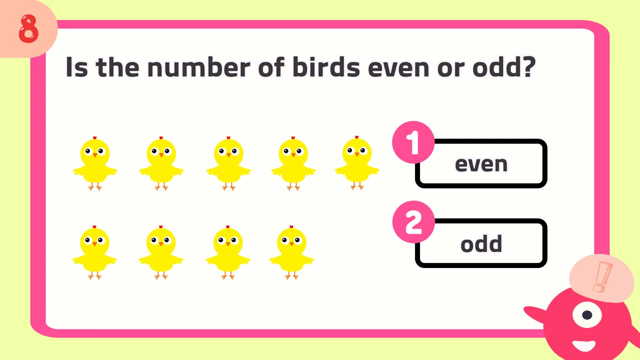 Is the number of birds even or odd? The answer is Odd. Number 7: Is the number of fish even or odd? The answer is Even. The answer is Odd. Number 8: Is the number of birds even or odd? The answer is Odd. The answer is.